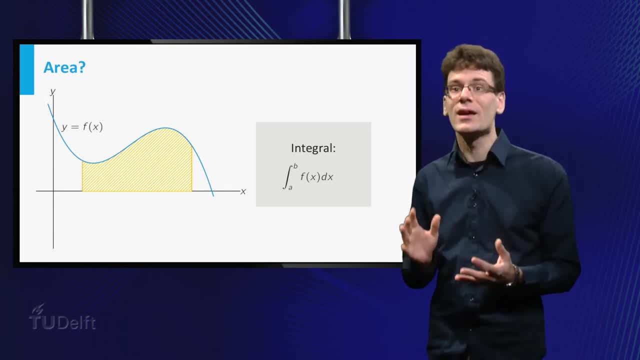 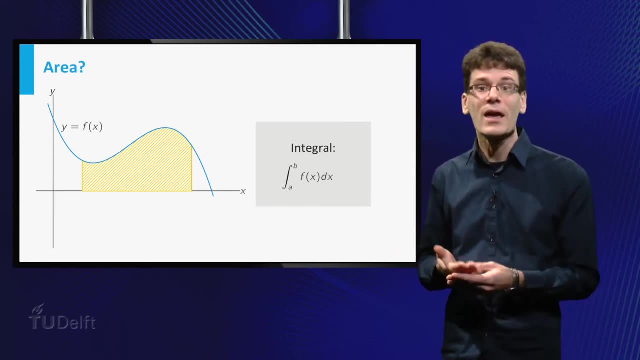 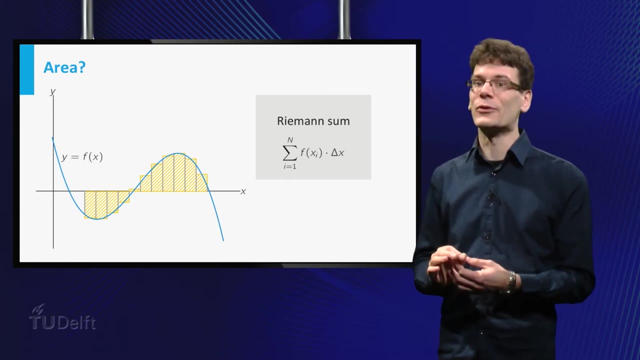 In this case, the area of the region is in fact, by definition, equal to the limit of the Riemann sum, And this limit is precisely the integral of the function over the interval. So in this case the integral is an area, But in general you have to be careful. 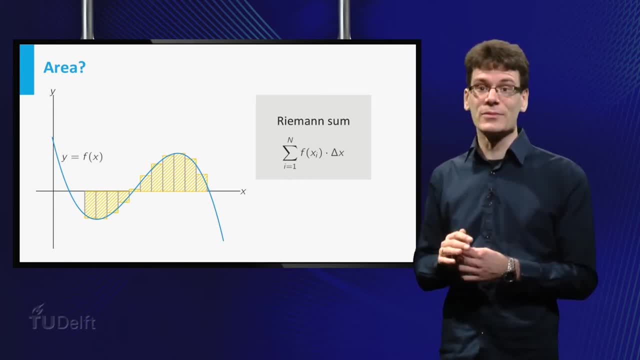 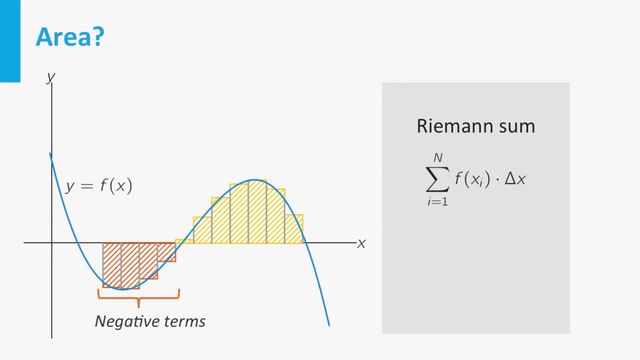 Problems arise when the function becomes negative at certain points. What is the interpretation then? Let us first look at the Riemann sum. At points where the function is negative, the corresponding terms in the Riemann sum will also be negative. Therefore, the Riemann sum represents the total. 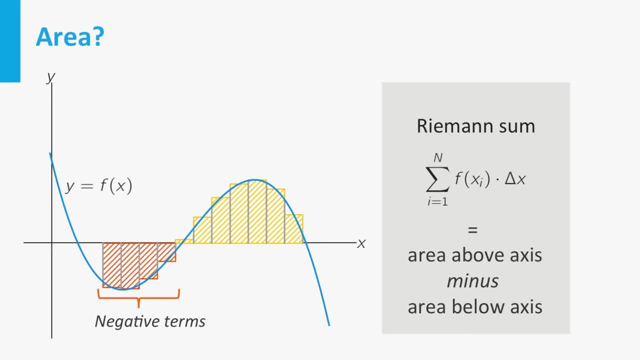 area of the rectangles above the axis minus the total area of the rectangles below the axis. Now take the limit to obtain the integral. The graph, the horizontal axis and the lines x equal to a and x equal to b enclose the region and the integral represents the total area b of the part above the horizontal axis minus. 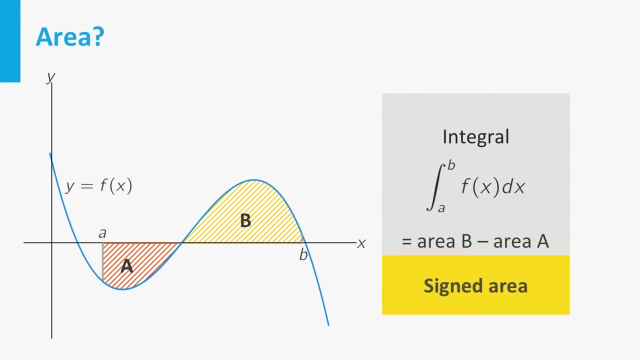 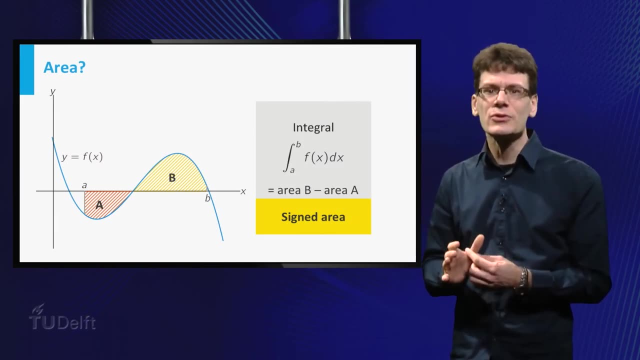 the area a of the part below the axis. It is referred to as the signed area of the region. You may wonder what the use of this signed area is Indeed. if you want to paint the region, it is of no use To know how much paint you need. you would. 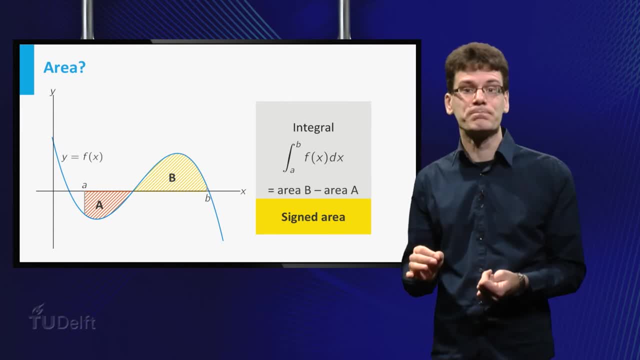 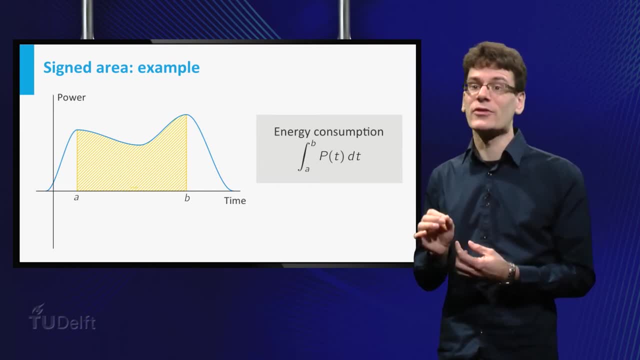 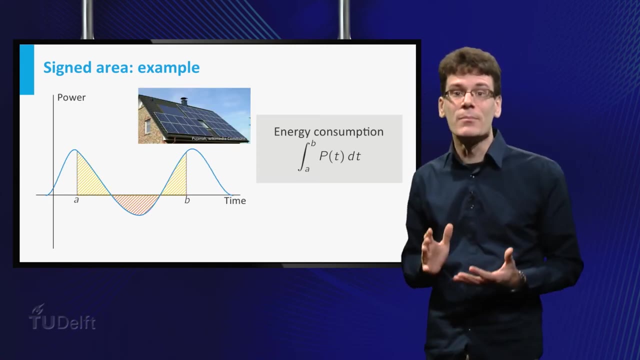 have to know the actual area, in this case a plus b. Think again of energy consumption. We have seen that it is equal to the integral of the power as function of time. How can power consumption become negative? Well, for example, if you live in a modern house with solar panels on the roof, 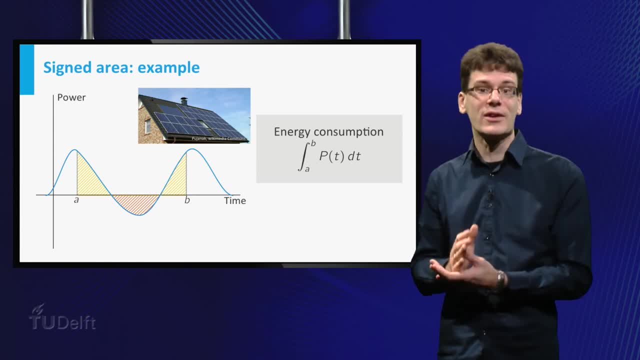 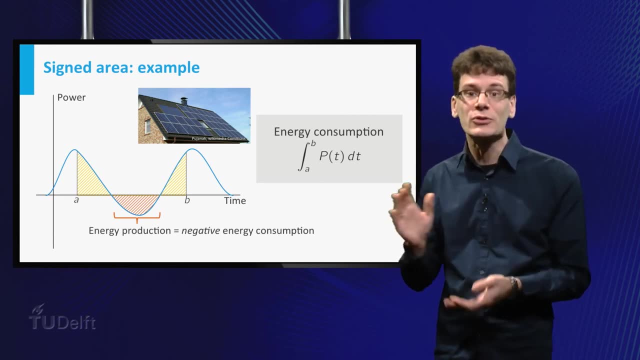 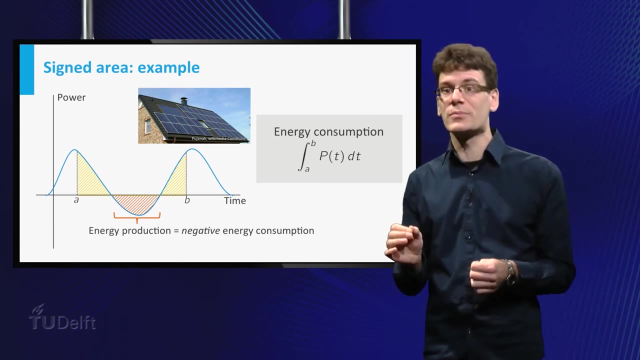 On a sunny day, the solar panels may produce more power than you use at that moment. The amount of power you deliver back to the electricity network is equal to the total area between the negative part of the graph and the horizontal axis, And to determine your effective power consumption you have to subtract this from the area between. 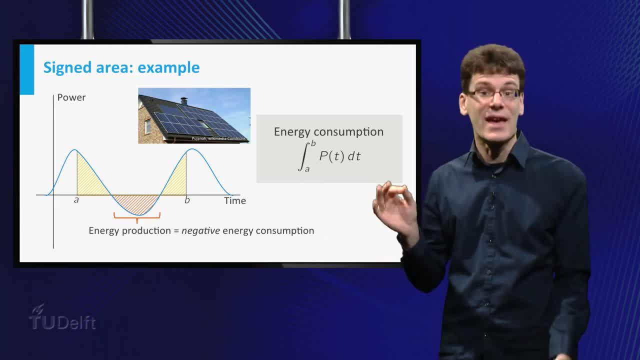 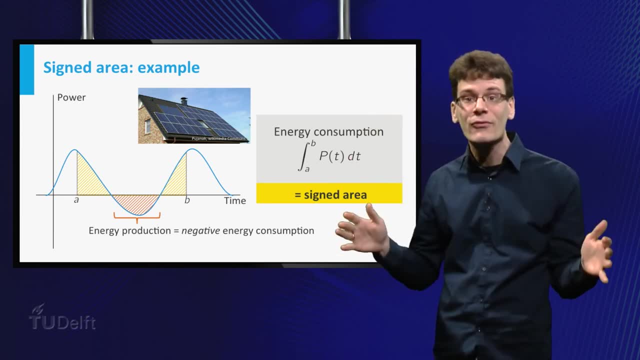 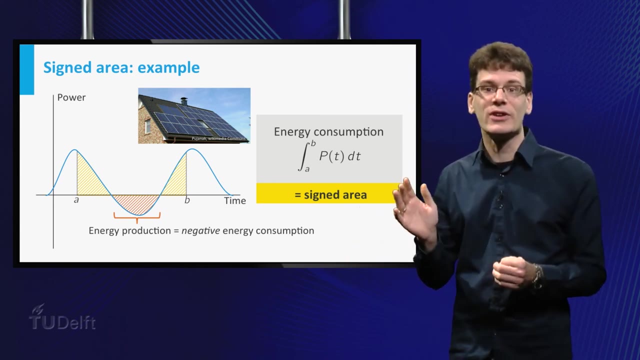 the positive part of the graph and the horizontal axis, That is, your total energy consumption is equal to the signed area of the region enclosed by the graph and the interval from a to b on the horizontal axis. QUESTION 4.. In fact, it is the aim of the Pret-a-loger project that we mentioned in the context video.